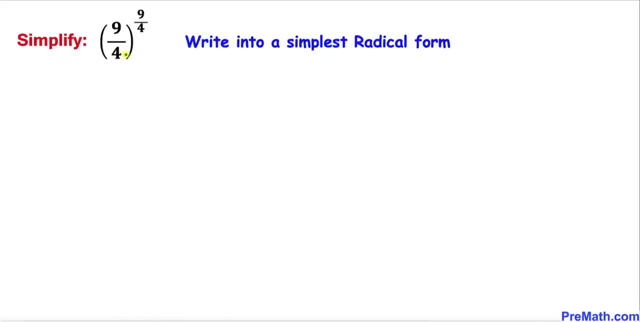 Welcome to PreMath. In this video, we are going to simplify this given exponential problem: 9 divided by 4, power 9 over 4.. In other words, we are going to write this given problem into simplest, radical form. Please don't forget to give a thumbs up and subscribe. So let's go ahead and get started with the solution. And here's our problem, and we are going to simplify it. Now let's focus on the base: 9 over 4.. 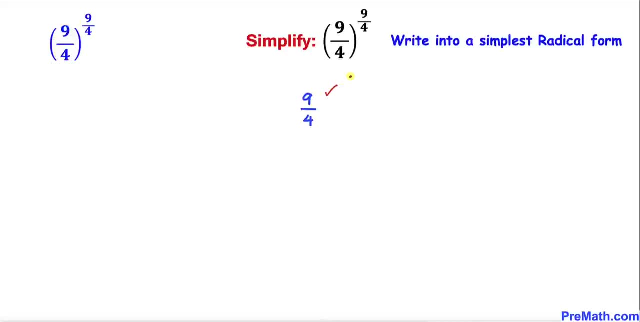 And here I have copied it down. and this 9 over 4 could be written as 3 divided by 2 whole square. Therefore, this 9 over 4 has been replaced by 3 over 2 whole square. And now let's recall this power rule of exponents. That means we can multiply out 2 times 9 over 4.. So therefore, we can write this problem as 3 over 2 whole square. 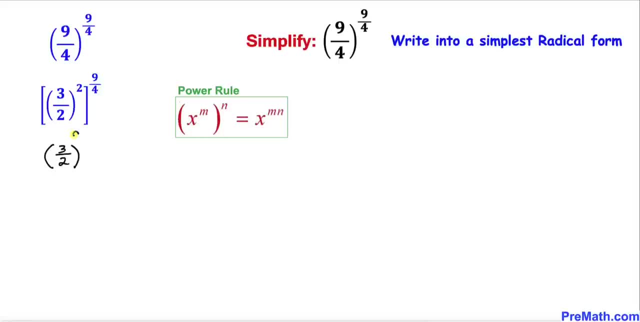 Whole power. 2 times 9 over 4 is going to give us 9 divided by 2.. And now let's focus on this exponent, 9 divided by 2.. And this 9 over 2 could be written as 4 plus 1 over 2.. And here I replace this 9 over 2 by 4 plus 1 over 2.. And now let's recall this product rule of exponents. So therefore this could be written as 3 divided by 2. whole power, 2.. 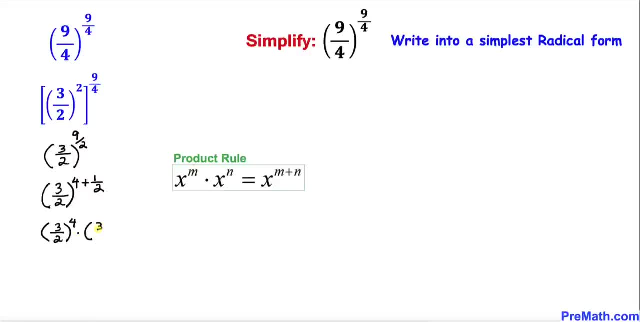 4 times 3 divided by 2, whole power 1 over 2.. And now let's focus on this part: 3 over 2, power 4.. And here, 3 over 2, power 4 could be simplified to 81 divided by 16.. Therefore, I can write this one as 81 divided by 16.. 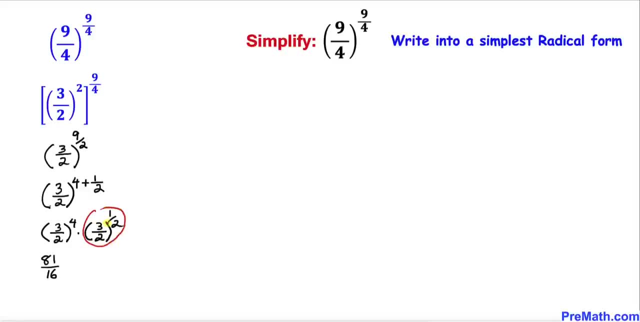 Now let's focus on this part: 3 over 2.. 4 times 3 divided by 2, whole power 1 over 2- could be written as, in radical form, square root of 3 over 2.. And in turn, this could be written as square root of 3 divided by square root of 2..